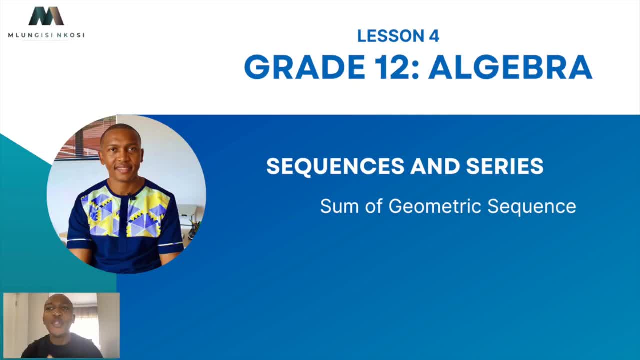 Good day. good day, everyone, and once again we are back together and welcome to our YouTube channel. For those of you who are new, please just make sure that you hit that subscribe button as well as the notification bell. And once again, for those of you who might need assistance in, 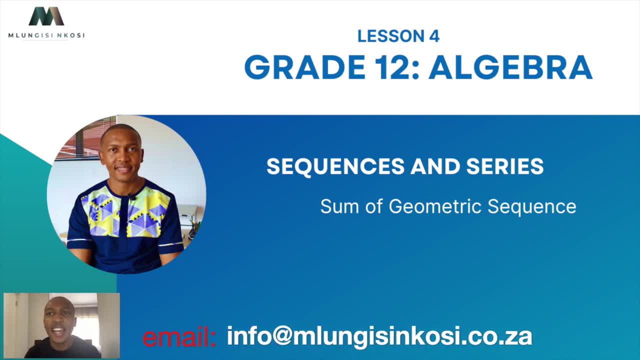 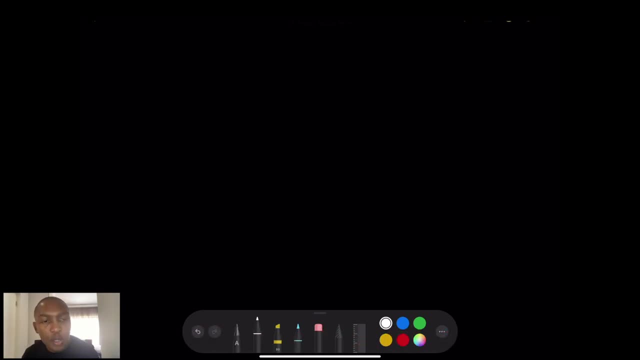 mathematics or physical science. let's be your plug, and our email address is info at mlungesinkosicoza. All right, so we are continuing on our lesson. Okay, so we're still looking at the geometric series or the geometric sequence. Now, in this particular case, I want us. 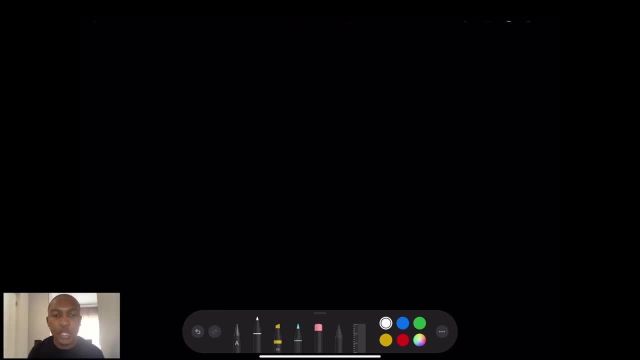 to look at the sum of a geometric sequence. Now there are two cases right that I'm going to mention. So when we take the sum of a geometric sequence, we have the formula. It says Sn is equals to A. Now this is going to be R to the power, n minus 1 divided by R minus 1.. Now this is for the case. 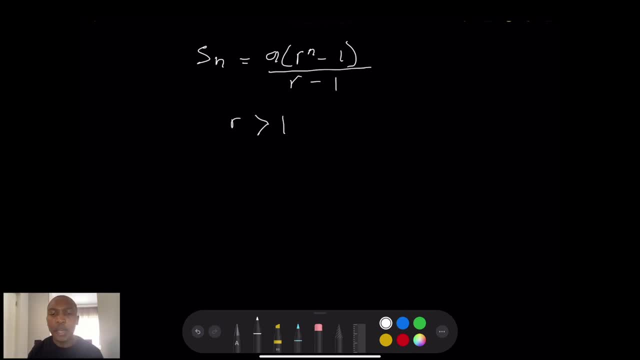 where R is greater than 1.. Okay, so this is the first instance. So whenever it is that we've got the common ratio- and of course I've already mentioned what A stands for as well as R, So when we've got the common ratio, in this case, to be greater than 1, then we can use 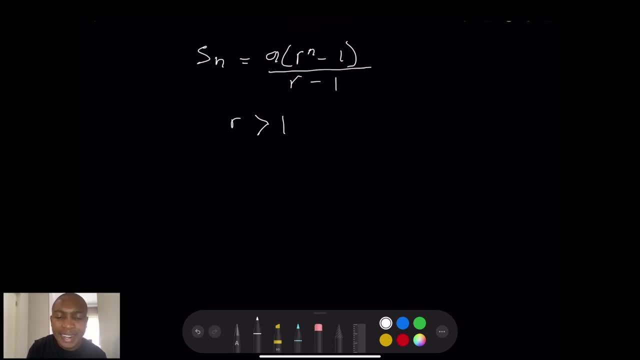 this formula. However, when we have R less than 1, then we use it. it's the same formula, but just you know, expressed differently. Okay, so this is where R is less than 1.. Okay, so sorry. 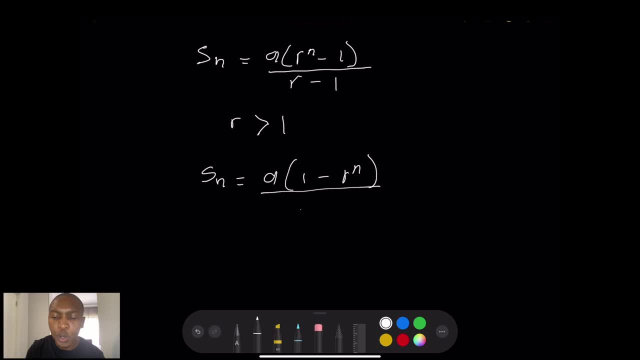 Um, so in this case, we're going to simply have 1 minus R. This is for all cases where R is actually less than 1.. Now, ladies and gents, what does it mean when R is less than 1 or where it's greater than 1, or? 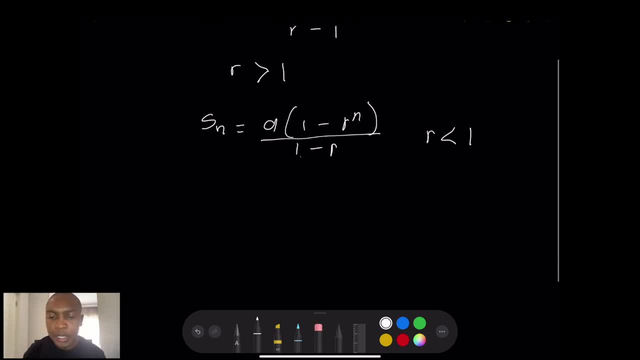 whatever the case may be right, I want you to keep in mind that R is the common ratio, which means that in this progression, what we are doing is that we are moving to the next term by multiplying by a constant. Okay, so that simply means: let's say we've got a progression, Let's say we've got. 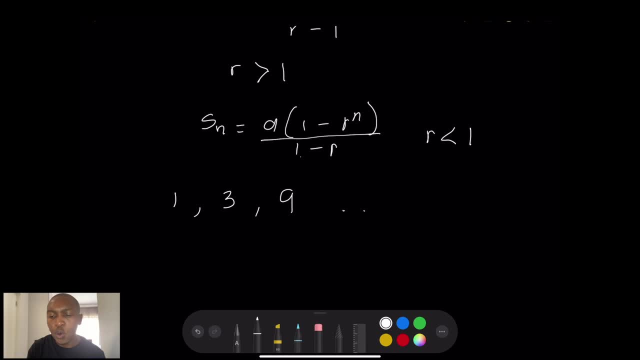 one, Three, nine and so on and so forth. right, So we know the value of A is one. We know R. I mean for you to move to the next term. what did we do? We multiplied by three For us to move to the next. 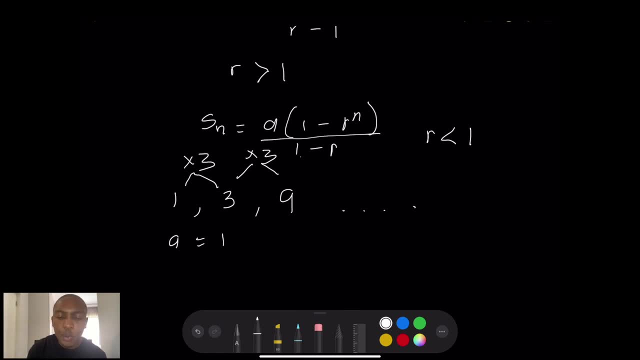 term. what did we do? We multiplied by three. So now when we look at our common ratio, in this case R is actually equal to three, of course. Now if I say to you, evaluate, you know the sum of the first 10 terms of the sequence. So now you've got the value of A. 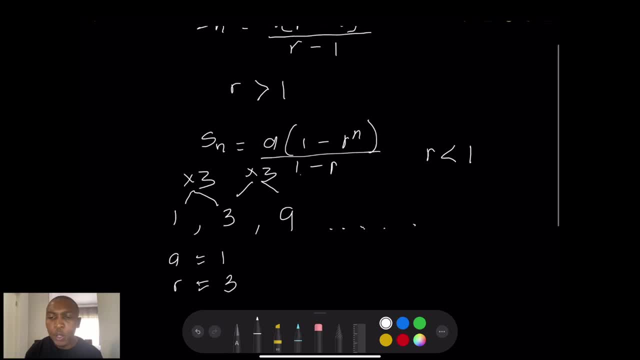 you've got the value of R, But now which formula are we going to use? You'll say to me: okay, well, R is actually greater than one in this case. So we're going to say: okay, so to get the sum of the first 10 terms. okay, so this is going to be S10.. Okay, this is going to be. 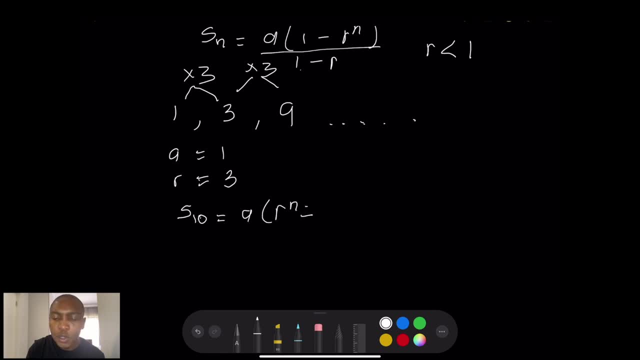 R to the power n minus one. okay, divided by R minus one. So, in fact, what you're now going to simply do is say: well, we know the value of A is one. we know R is actually equal to three. So this: 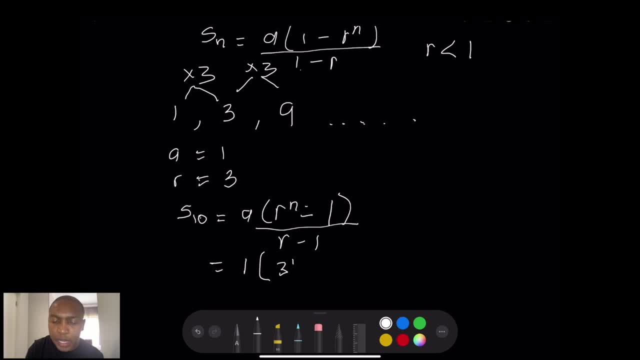 is going to be three to the power, 10 minus one divided by now. I'm just going to pull this up a little bit. Okay, We said that's three minus one, So this is how simple we'll get the sum in this particular case. 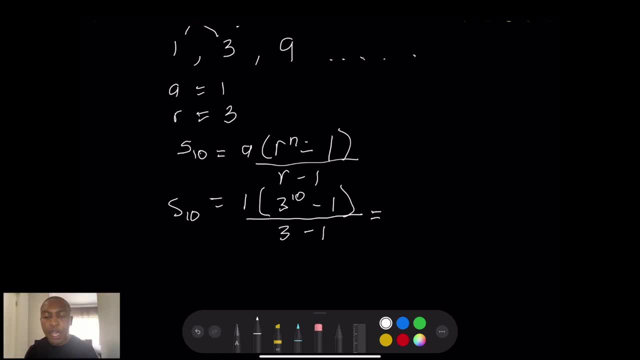 I'm just going to throw in some terms there. All you need to do is just put this in your calculator. Let me do that quickly. If you can try and do it as quickly as you possibly can, that would be really helpful. So this is three to the power: 10. Okay, minus one. 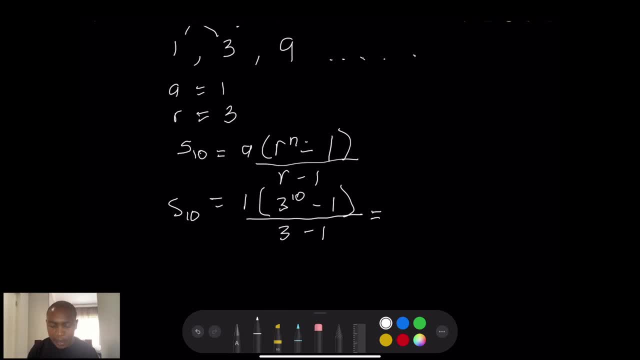 Just be careful when you are pressing on your calculator, especially when you're dealing with an exponent. okay, Make sure that you put on that cursor. All right, so the value that I get there is 29.. Perhaps I should download a an emulator so that I can be able to show you. 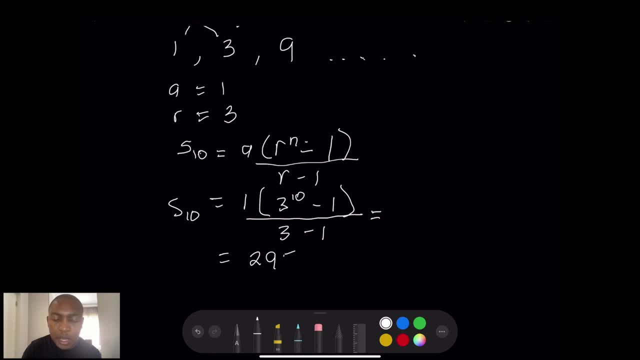 every time I calculate. So in this case, that's twenty nine thousand five hundred and twenty four. Now, what you realize here is that every time you're making a calculation, you'll see that the value gets bigger and bigger. Now we call this a divergent, you know series. 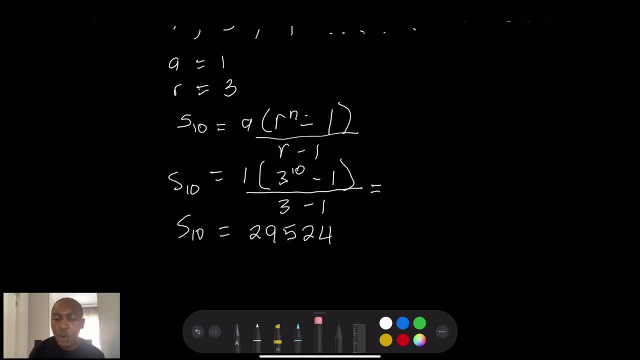 OK, we call it a divergent series. What do we mean? We say the further we move, you know, away from our terms, or the further away we move from you know. let's say that's one, that's three, that's nine. 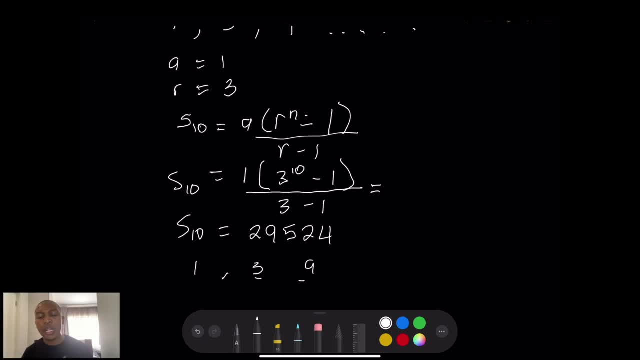 So obviously, every time you are telling up, you are counting up the sum, the number simply gets bigger and bigger. OK, of course it does make sense. But what it also means is that in this sequence, if I were to kind of draw it as a, you know, you can imagine that the progression, the further you go, towards infinity right. 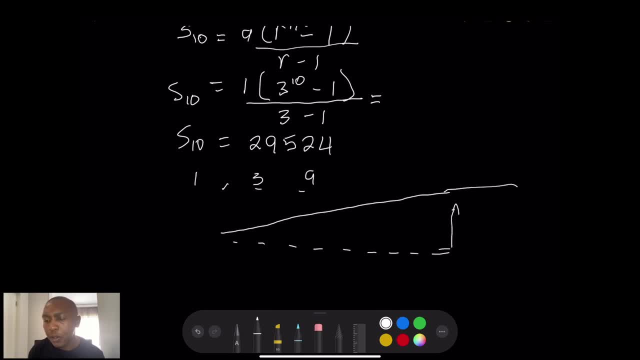 The numbers simply keep surging up. OK, keep going up. So we say it's a divergent sequence, Right? However, suppose we were to have a situation. Let me just Make a progression there. OK, say, we've got, you know, let's have one, one over two, one over four, and so on and so forth. 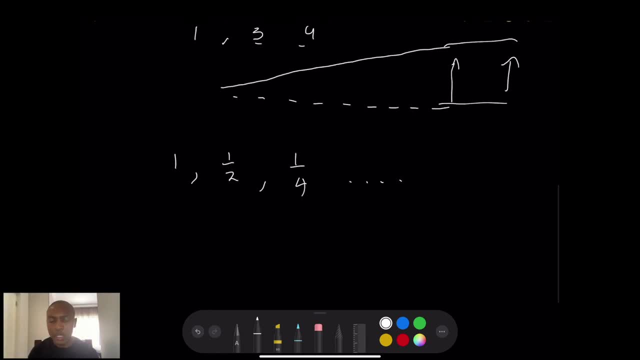 Now, here we've got another sequence Right. But in this case, what would be our value for R? Of course, you're going to find the common ratio. How do we find the common ratio in this case? Or well, is it? 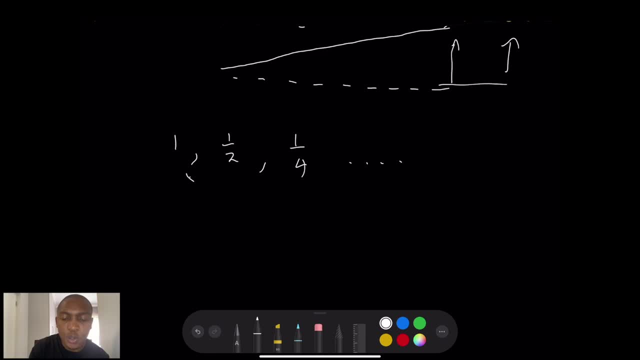 Do we have a common ratio? That's the first thing that we should check. So let's see, how do we find the common ratio? We said to do that. you simply say T2 divided by T1.. So let's see, what do we get? 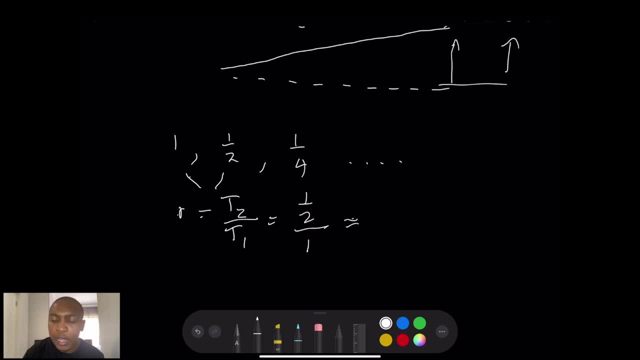 We will get one over two divided by one, And that gives us one over two. That's a half right, But would that be the same if we were to take T3 over T2?? Of course we're not going to waste time. 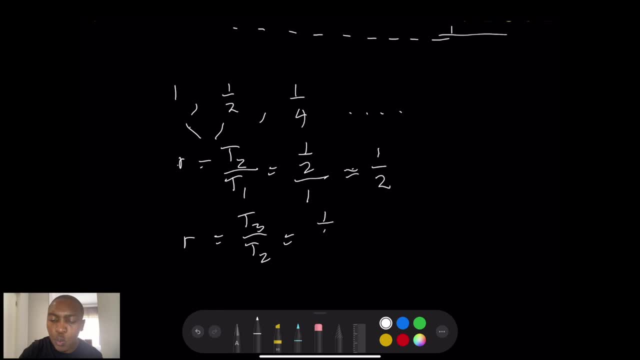 We've already covered this. OK, so you're going to say: this is one over four, divided by one over two. Now I honestly want you to be very careful when dealing with fractions, And perhaps what I will do is just have a lesson on fractions by itself. 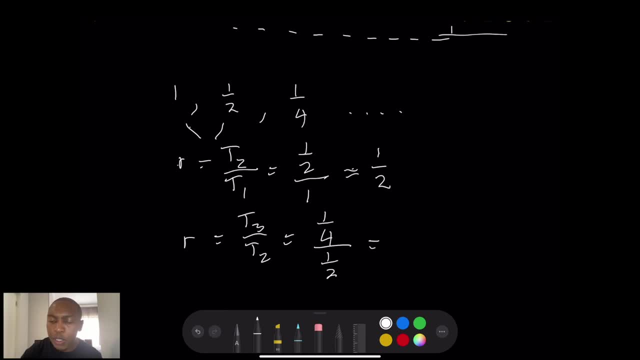 OK. so when I'm dealing with this fraction, I'm going to simply say: OK, so I've got one over four Divided by Now. I'm going to simply have divided by one over two and express it like that: 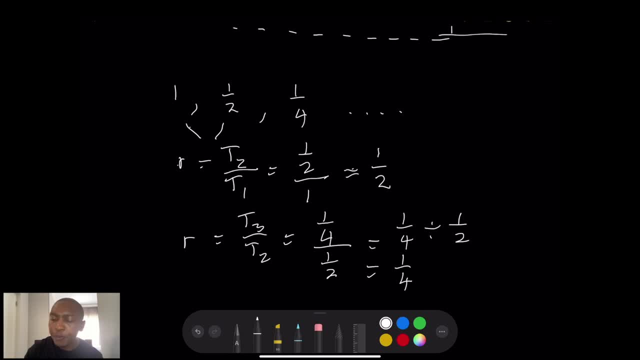 But remember when I'm dealing with fractions. OK, I can convert that division sign into multiplication, But in order for me to do that, it means that I need to now invert the other fraction. OK, so that now becomes two over one. 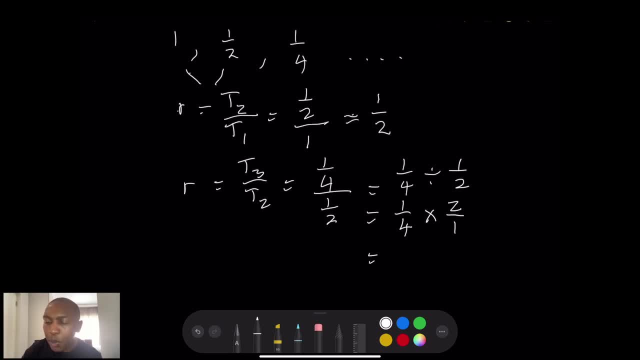 Please keep that in mind. So what I'm going to have is one over four divided by, Multiplied by two over one, and I can simply multiply the numerators: One times two is two and four times one is four, And you'll see, two goes into itself once and it goes into four twice. 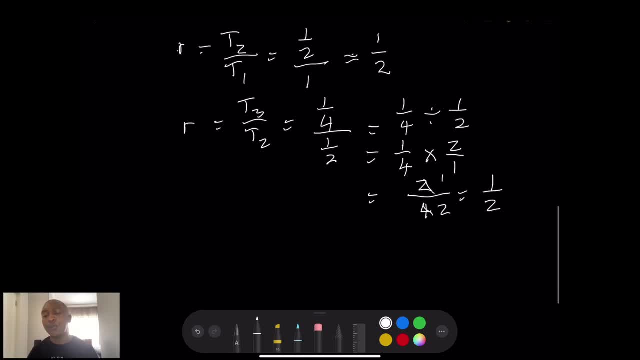 So this is the same as one over two. So definitely we've got a constant or a common ratio, in this case to be one over two. Now, if I were to ask you to calculate the sum Of the first ten terms, OK, so as ten. 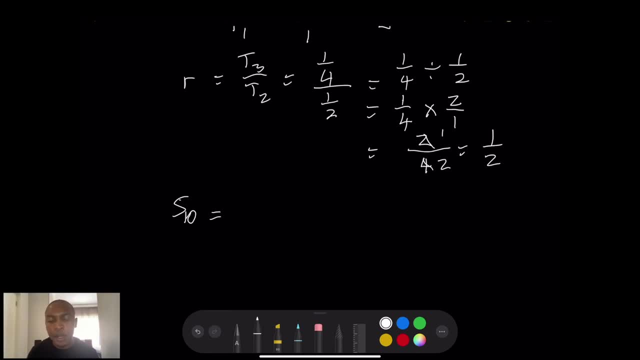 For this one here. So you'll say to me: OK, the value of R is less than one. OK, meaning that it is, Yeah, it's less than one. So what we're simply going to say is a That's one minus R, to the power N. 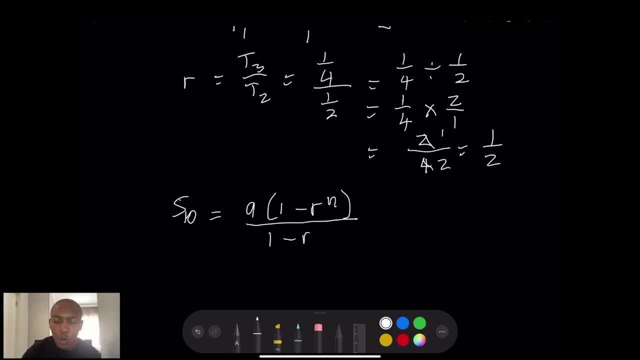 Divided by one minus R. So all we simply do is just to substitute Once again. our value of A is one, OK, that's one minus. We said R is one over two. OK to the power N. And we said: this is the first ten terms. 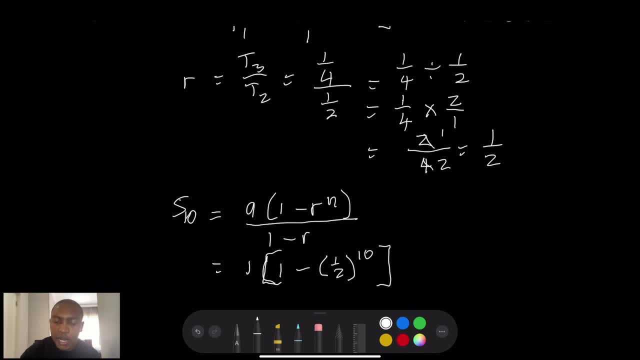 In fact, let's do this. Let's put that in square brackets divided by Now. this is going to be one minus one over two. OK, so please keep in mind- Very important for you- every time that you make a calculation, to be mindful whether R is greater or less than one. 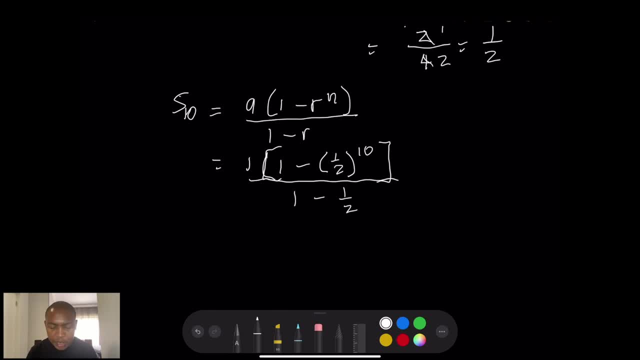 OK, So I'm going to quickly just put that in my calculator there. OK, so we've got. this is going to be one minus. OK, and I did say: for your benefit in future, What I'm going to do is just download an emulator so that you are able to. 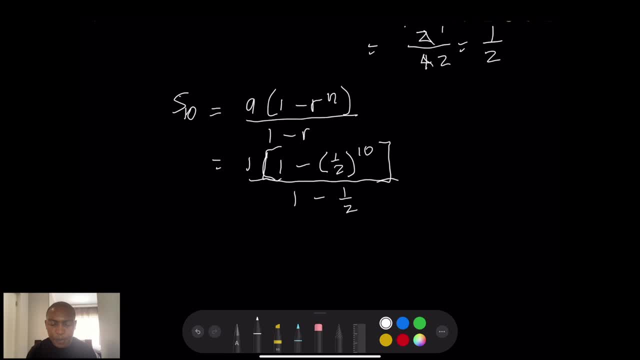 You know to see that as I calculate, OK, and then divided by one over two, OK, right, One minus one over two, OK, and I get a value there, Right, You can express it as a fraction. The value that I got there was one zero two. three over five twelve. 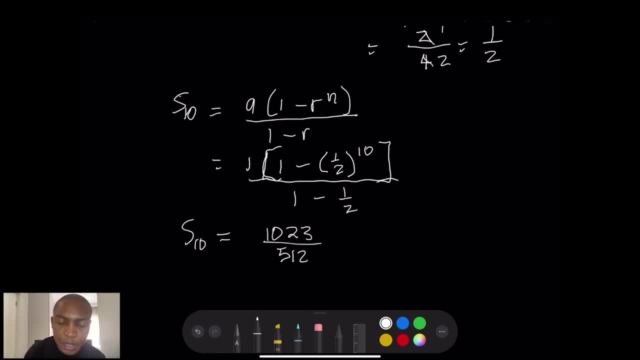 OK, So this is the sum of the first ten terms OK, And Which is approximately equal to one point two, Because it's it's one point nine, nine, eight, So this is approximately equal to two. OK, Right now, Ladies and gents, what I want to quickly do is I just want to quickly jump into talking. 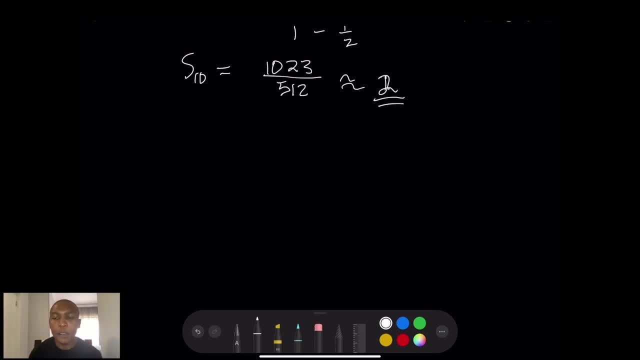 about The sum to infinity. OK, Now We say that when are the value of R is less than one? We say: this is what we call a convergent series. It converges towards a particular you know, it converges towards zero. in that case, 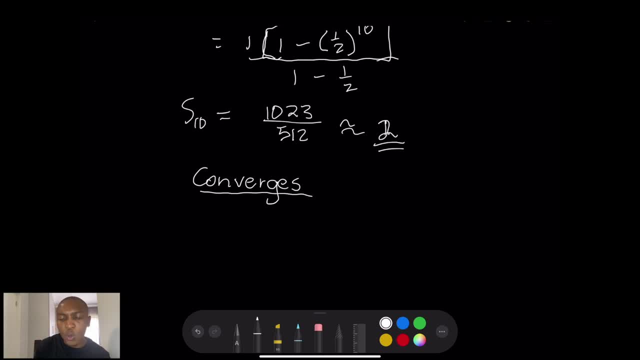 OK. So it means that the further you go- now I want you to think about it- You start with a number. Let's say you OK, Let's. let's take a progression. Let's say you've got eight, Then you've got four. 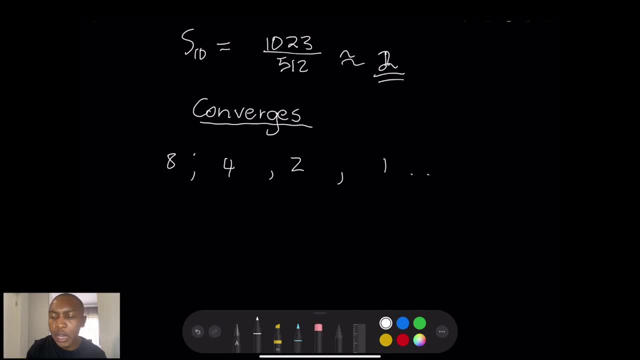 You've got two, You've got to one, and, and you keep going. What's happening in this progression? It is definitely a geometric progression, But the difference is that the numbers are getting smaller and smaller and smaller. Now you can imagine that the further you go, towards infinity. 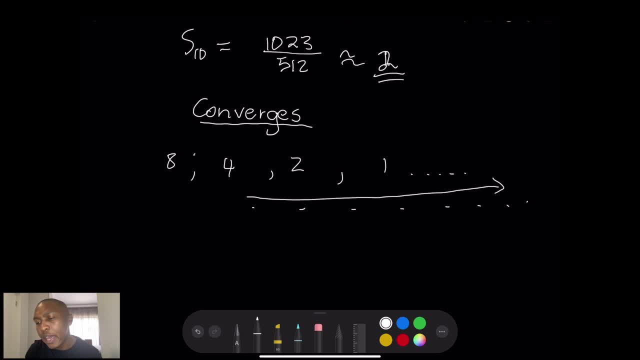 They Get small, that you actually end up, you know, with a number as close as possible to you know, to zero, right? so meaning that you can actually find out what is the actual sum to infinity. okay, so what I want us to quickly do is: let's talk about the formula of the sum to infinity, okay. 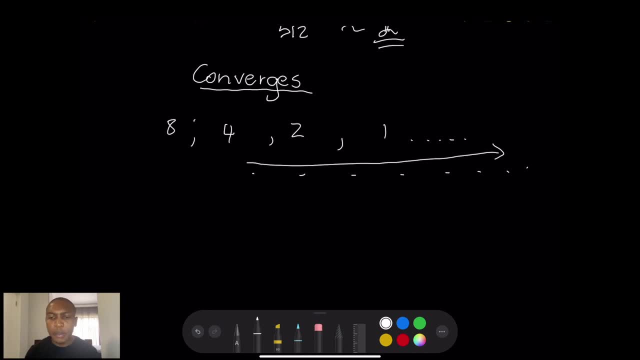 okay. so let me actually take the very example that I made here so that I can illustrate using it. okay, so if I have got this particular progression, it means that as I move towards infinity, the numbers get so small and small and small that they actually move towards zero, and 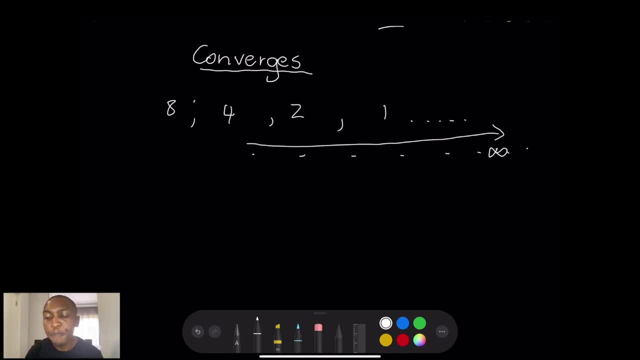 ultimately, you can actually get the sum to infinity. if I could, if I had the time, I would actually, you know, illustrate this to you better. okay, so that you can see it all. right, so what we're going to do is right, right. what is our value for a? our value for a, in this case, is 8. okay, and our value? 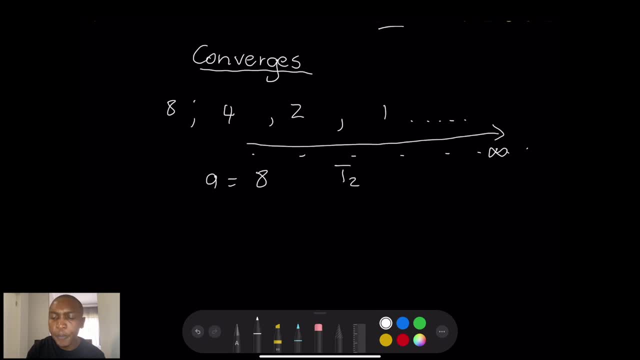 for r, if you take t2 divided by t1, this is going to be 8 divided by 4. sorry, actually the other way, sorry about that. okay, so that's 4 divided by 8. so that's 4 divided by 8, and of course, you can. 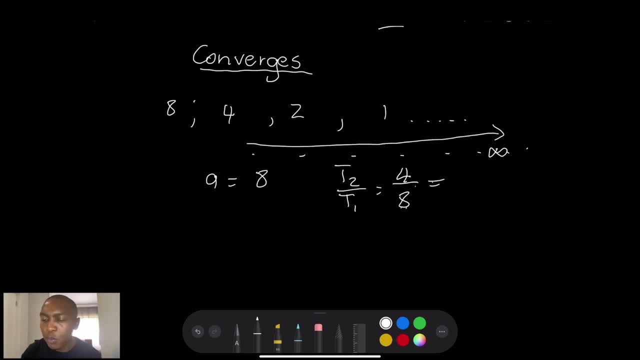 do the same with t3, just don't want to waste time with it. so in fact, that's 1 over 2, right, okay? sorry that I'm using the same common ratio again. okay, so what I want to do is talk about sum to infinity. so I've already established that my value for r 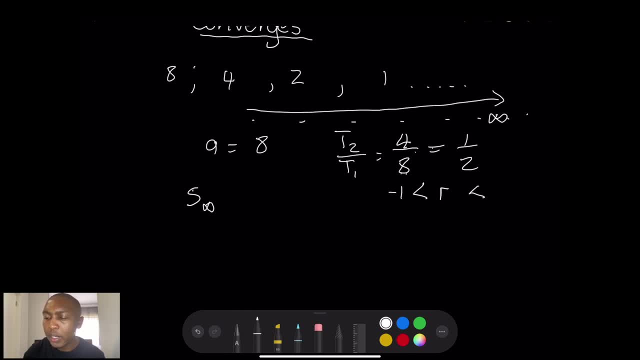 is between minus 1 and 1. now, remember, once this is the case, then we say that our series or our sequence is convergent. we did say that. right, okay, is convergent, remember it converges. what that simply means is that you know, as you get the numbers, they get smaller and smaller. 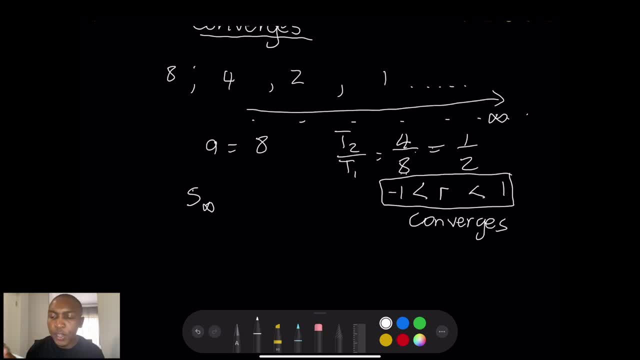 and they sort of lean more towards a specific number, in this particular case zero. okay, so now what we say is: the sum to infinity is simply going to be a divided by 1 minus r. now I could show you where this comes from, but that's another discussion for another day and that will have a 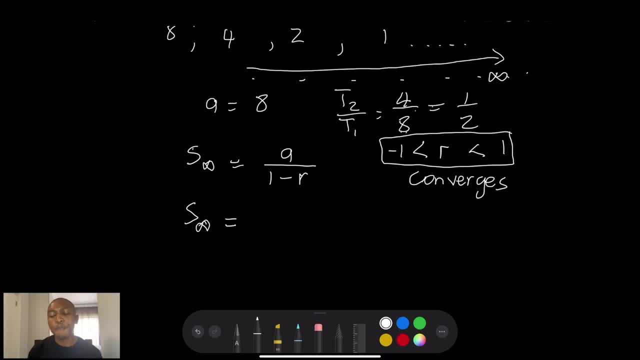 different purpose all by itself. so what we're simply saying is that when you calculate the sum to infinity, you can only do that for a convergent series, okay, meaning where r, the value of the common ratio, is less than 1 and it's greater than minus 1. so let's find out. 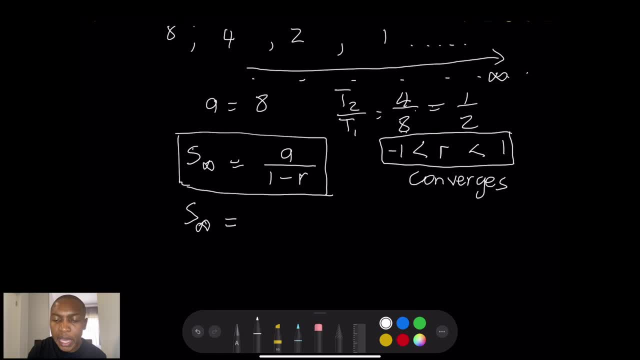 for this one. what would be the sum to infinity? so that would be a. what is our a value? a value would be eight. okay, and what is our r value? we just found out that our r value would be 8. okay, now is 1 over 2, so our sum to infinity this will be 8 divided by 1 minus 1 over 2, that's 1 over 2. 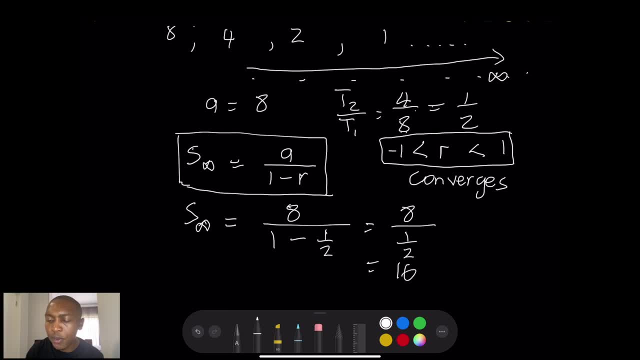 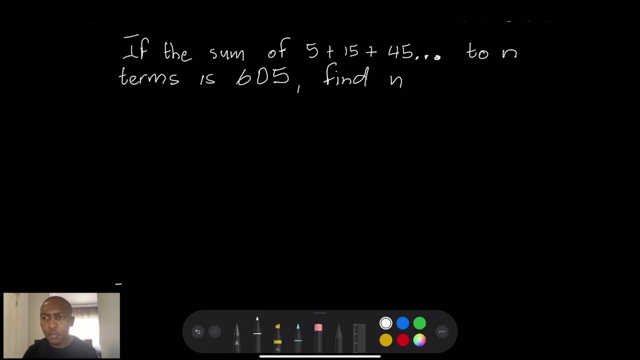 and this is simply going to give us a value of 16. so it means the sum to infinity for this particular question is 16. okay, all right, let's take this as our next example. let's say, if the sum of 5, 15 and 45 to n times, 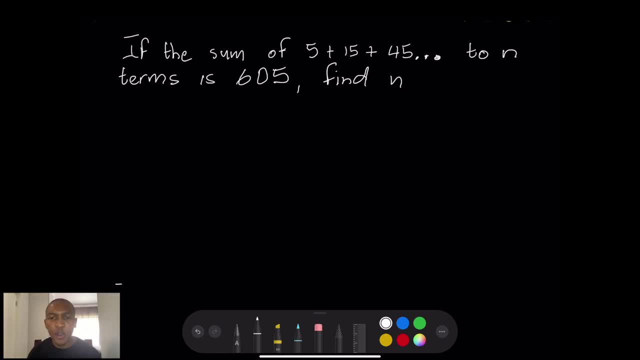 is 605. okay, find the value of n. so there are two things that we need to establish here. what is our a value? so, without any waste of time, we know our a value is 5. what is our r value in this case? so that's going to be. 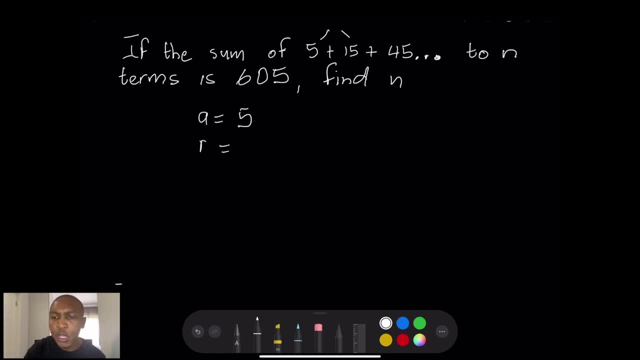 um, so to move from the first to the second term, okay, you realize, there we've got 15 divided by 5. that will give us 3, and of course, 45 divided by 15 will also give us. so we're taking term 2 divided by. 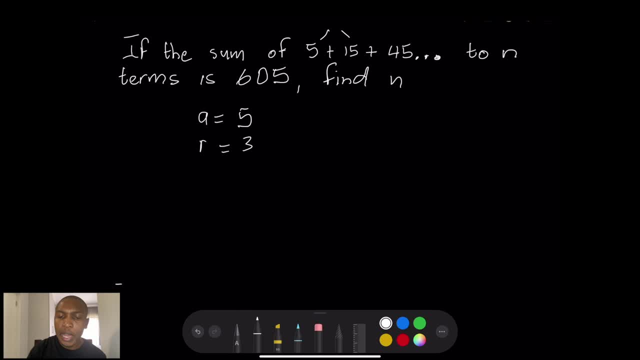 term 1 as well as term 3 divided by term 2, and that gives us a value of 3. i'm not going to waste time with it. okay, so now we want to know how many terms will give us a sum of the sequence? definitely, 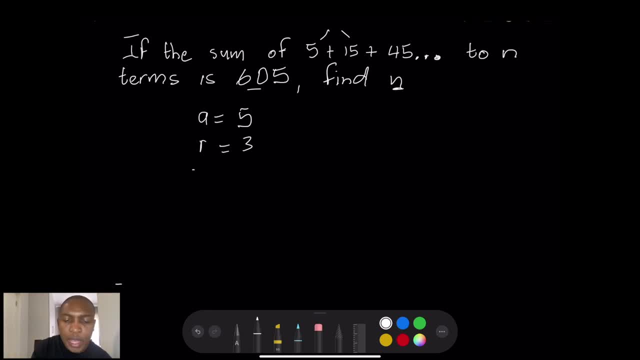 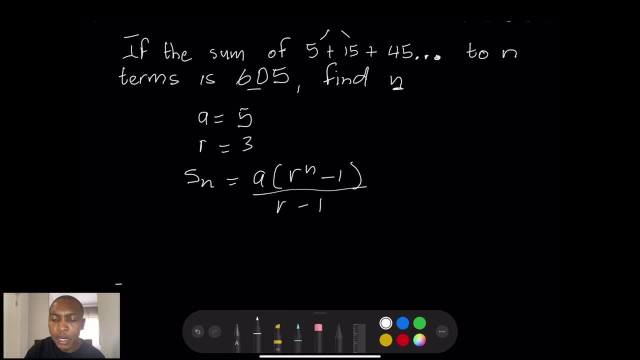 n minus 1 divided by r minus 1. so quickly, let's do that. so this is going to be 5. okay, so that's three to the power n minus one. okay, divided by three minus one, and all of this is equal to six, oh five. so now we have to kind of 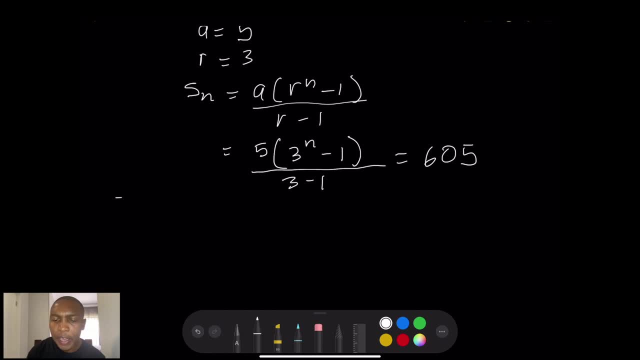 work with exponents, we have to work with fractions, and and so on and so forth. so in this case we've got um, okay, let's simplify this. so this is five over three, okay, sorry, five over two, and three minus one there. okay, three minus one gives us two. um, yeah, this technology right, so three uh. 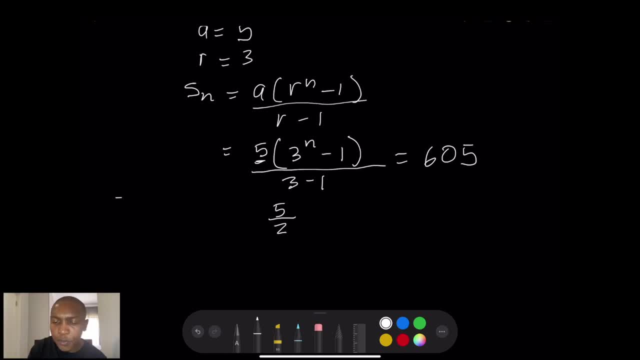 five. there's a five there. uh, divided by uh, three minus one gives us two. but all of this is multiplied into three to the power n minus one. okay, is equal to six. oh, five, now, uh, if i may quickly just show you. so we've got a. 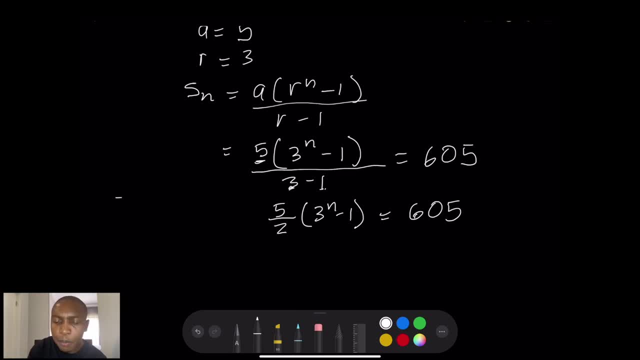 coefficient, the fraction as a coefficient there. so all i'm going to simply do is just multiply by the inverse of that fraction. uh, that's two over five. but remember, what i do on the left, i have to do on the right, and the reason i'm multiplying by two over five is that, uh, those will cancel out. 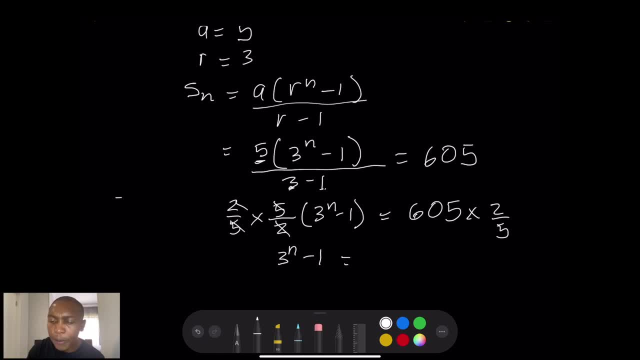 so i've got three. add to the power n minus one, okay. so i'm going to say six or five multiplied by two over five, um, and i get 242, okay. and if i take the one to the other side, remember we cannot add it to the- 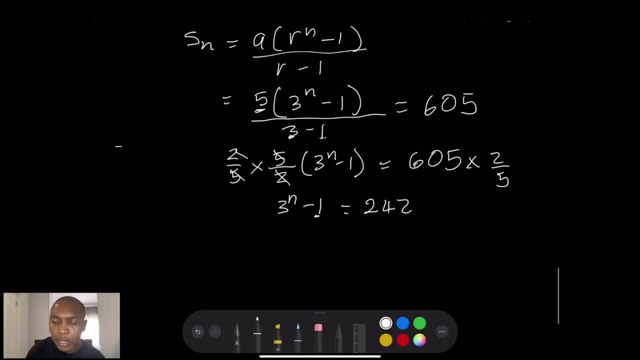 three to the power n. they're unlike terms, uh, in that case. so we're going to have 3n. if i take it to the other side, it will be 242 plus one, so i'll have 243. okay, so, um, either you can use logarithms. 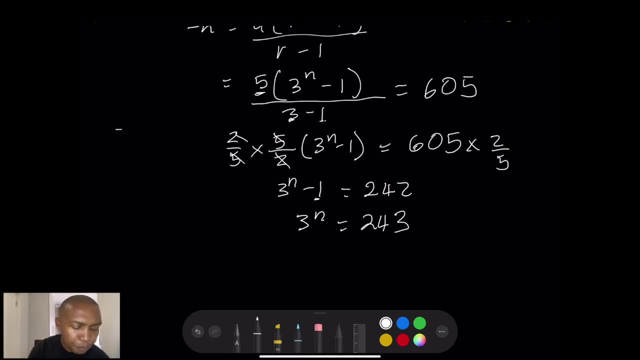 or we can just simply find out. okay, um, you know, um, what are the factors, or rather, um, what is the power of three that would actually give us a, a 243 right. so, um, to be quick about it, you can just simply introduce logs and say: well, this is going to be log of 3 to the power. n is equal to the log. 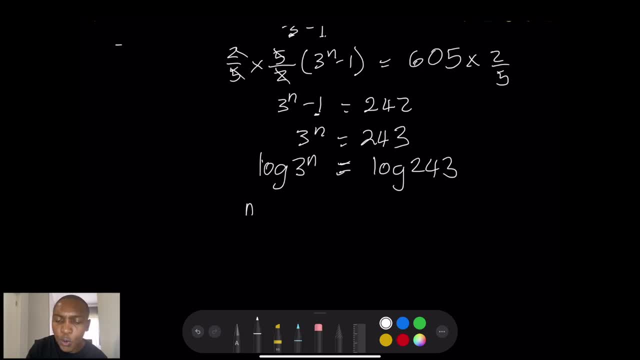 okay, um, of course the law of logarithms says: okay, if i've got a, a, a power there, it can jump down that jump down rule. so n log of three is equals to log of 243 and you can divide both sides by log of three. uh divide by log of three. uh, so a value for n right, let me do that quickly. so log of 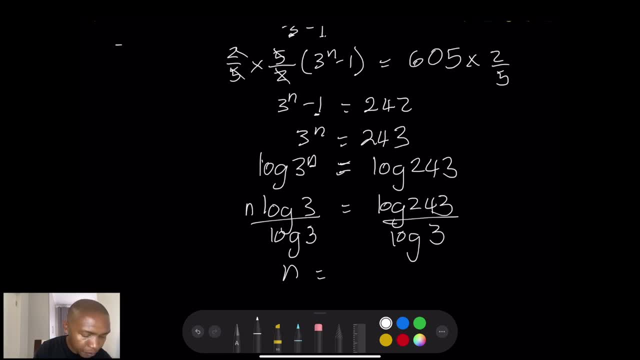 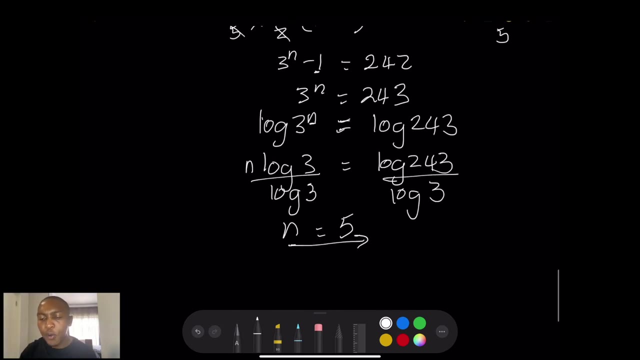 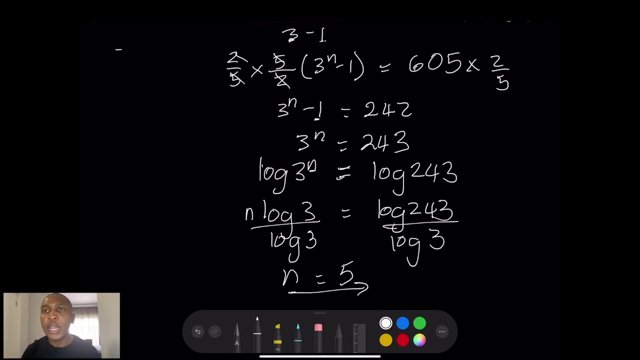 200, 43, uh, and i'm going to divide that by log of three, okay, and my answer is five. so it means that the sum of the first five terms will actually give me, uh, that value of uh 605.. i hope that makes sense, ladies and gents. um, and i just want to make um. maybe just one last example.